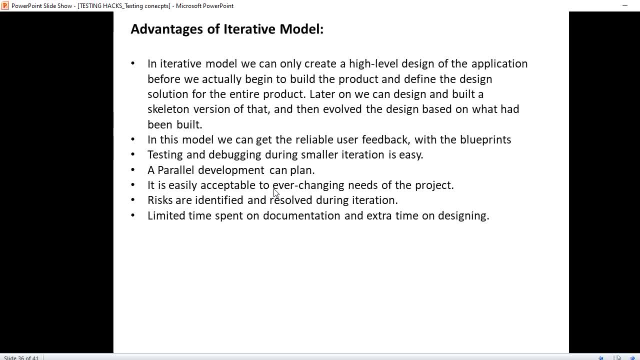 design solution for entire product. Okay, Later on we can design and build a skeleton version of that and then evolve the design based on what had been built. So as this advantage says that though a skeleton will be designed, so where in very first the skeleton will be designed? 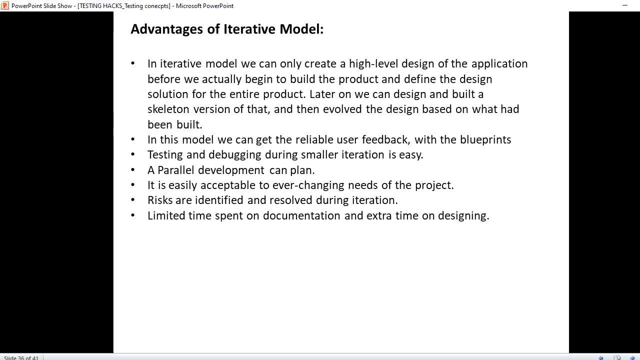 designed. I mean the look of the, how it looks like and all. all this will be designed first and then that will be evolved to next phases. okay, in this model we can get the reliable user feedback with the blueprints. as we have already mentioned that this skeleton will be prepared first, right, so with 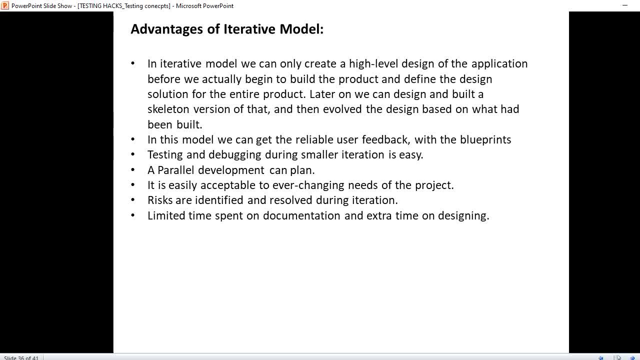 that a skeleton. the customer will provide the feedback any improvements is required on. based on that feedback will be collected and then the then the changes can be done. right, because it is initial stage, only a skeleton will be prepared. testing and debugging during smaller iteration is easy. okay. so since 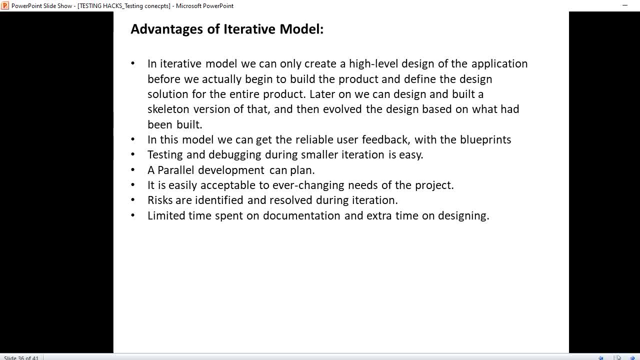 it is a smaller iteration so it is easy. a parallel development can plan. so during this phases a parallely development can also be planned, because the skeleton is getting ready here and the parallely, the development, can also happen. you know, in that way it is easily acceptable to ever changing needs of the project. so since I 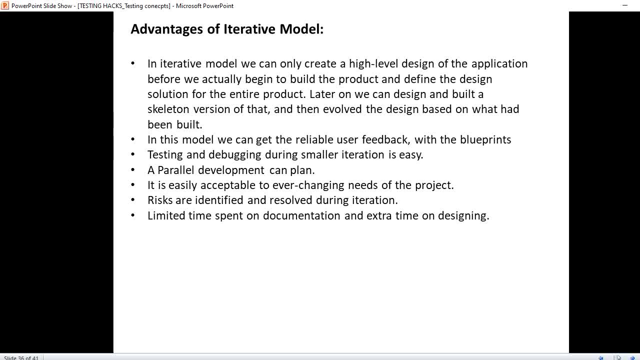 have already mentioned that, based on the feedbacks, we can also change the requirements, right? so since the product is not ready yet, it is just as a small division, right? so it is easy to handle the requirement changes. also, you know, the risks are identified and resolved during the iteration. okay, limited time. 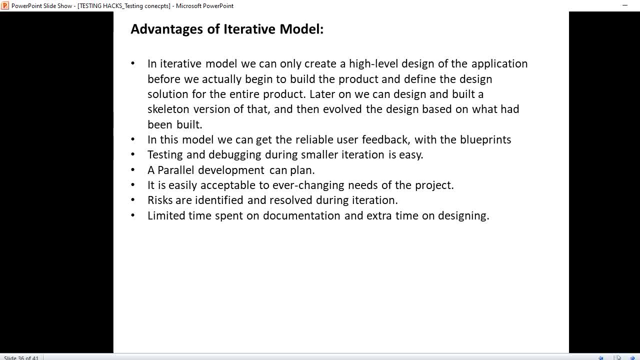 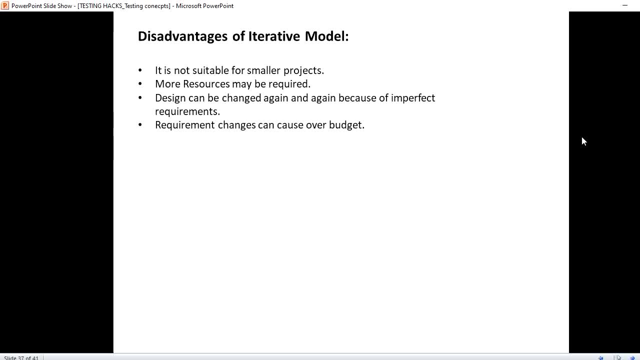 spent on documentation and extra time on designing. okay, so these are the advantages of iterative model. when it comes to disadvantages, it is not suitable for smaller project. if the project is smaller, then I think this is not a best suitable model. more resources may be required, since it the with the